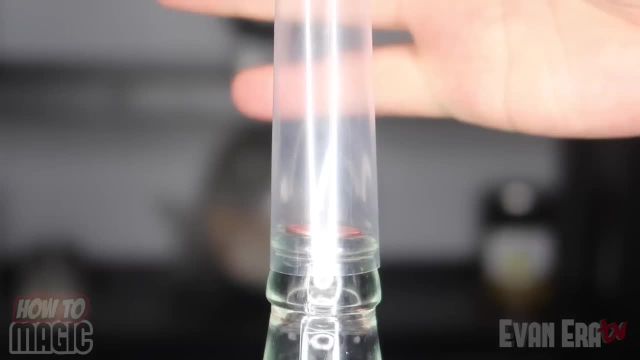 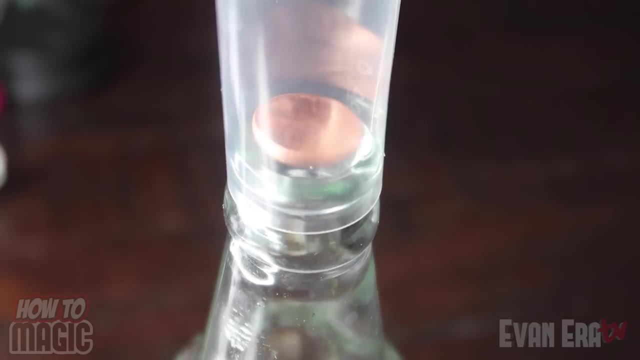 You're on And when you drop the marble, this is what's happening inside. It's flipping the penny up, The marble's dropping in and the penny's falling right back down on top. This is the perfect one to do at home. 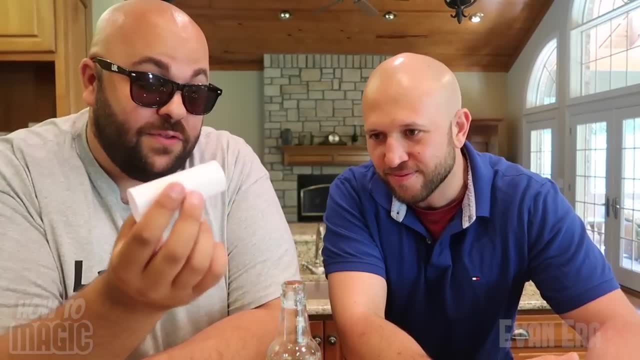 Especially on kids. Oh yeah, totally. This is a really easy one too. All you have to do is drop it, and it pretty much does the magic for you. Let me try it. Let me try it. So put the penny on top. 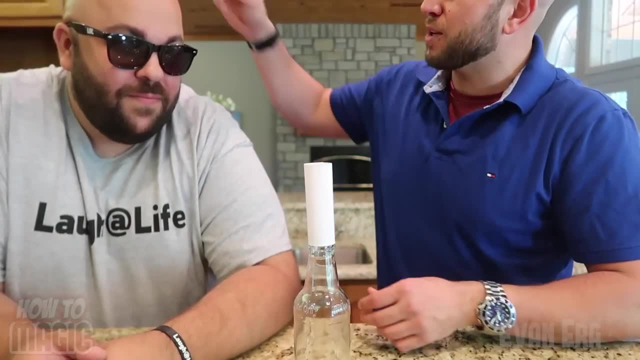 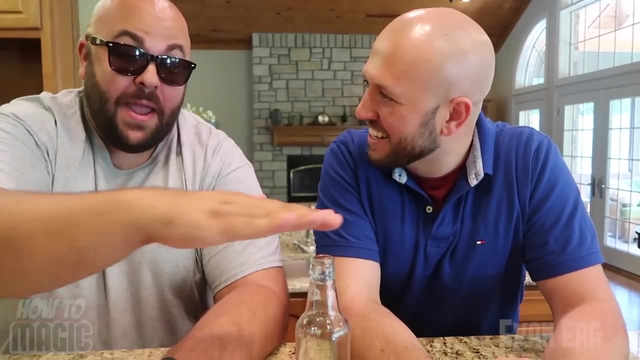 Yeah, So easy. even the kid can do it. Right there, I'm going to do the magic juice. There you go. Look at this Now. make sure you immediately pull this off And show them that the penny's like still flat on top of the bottle. 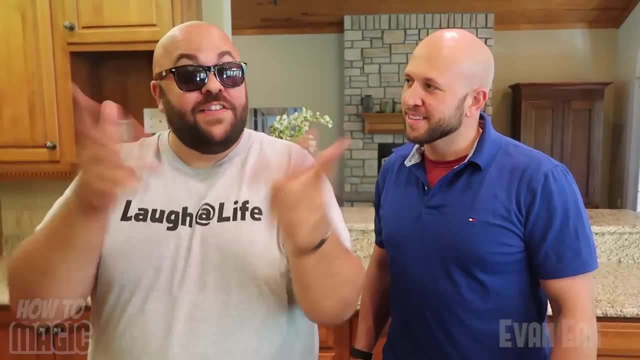 And that is how you do the magic marbles of the coin trick. Okay, this is another easy one that you can do at home. All you need is a sheet of paper. Check it out. All right, Veronica. so I have a rolled up piece of white paper here. 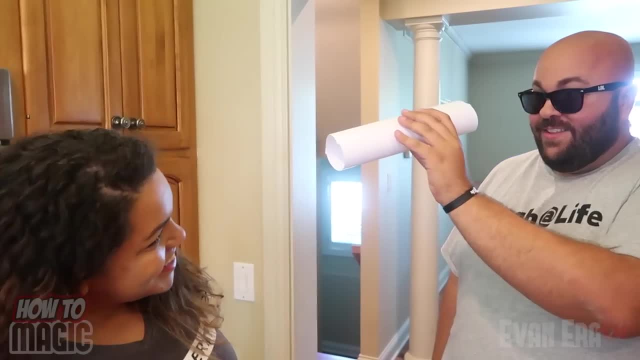 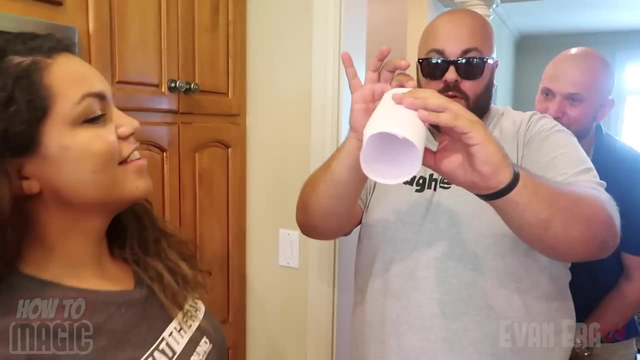 This is a piece of white computer paper. you can see through the middle. It's empty. Yeah, All right, watch, Nicely made. If I give it a nice magical wave like this, look, You can see this happen. Where did you get that? 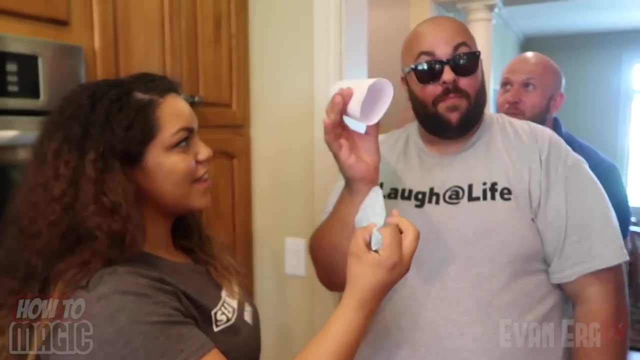 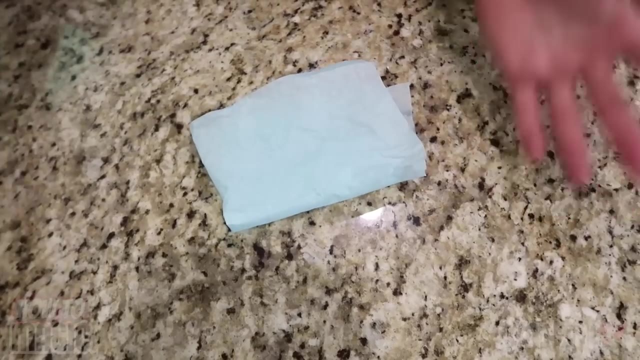 Cool, right, Yeah, Where did that come from? Here's the secret to this amazing magic trick. Okay, so here's what you need for this trick: Two pieces of paper, some tape and a piece of tissue paper. So your first step is to take one of the pieces of paper and you're going to roll it, just like this: 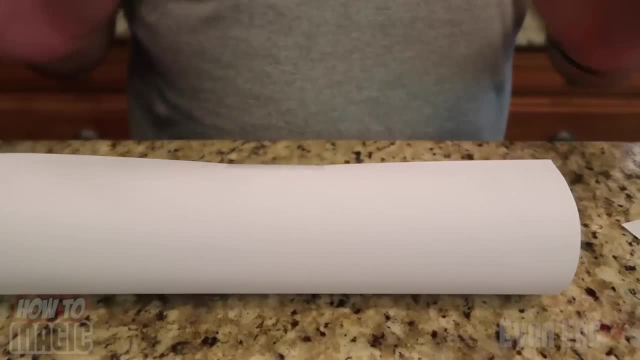 I'm going to put a piece of tape right in the middle, just like that. Now, you want this to be perfectly even like this, So you want to put a piece of tape on either end too, just like that, and on the other end as well. 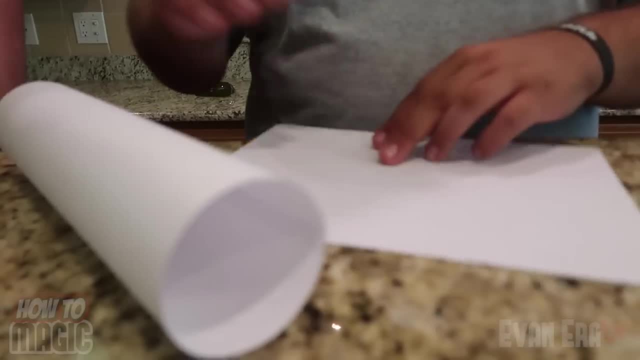 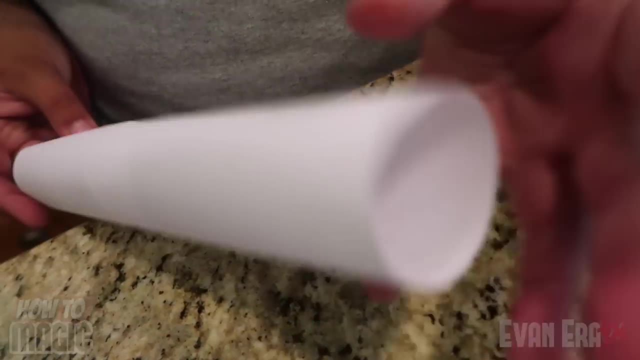 So that is one piece of paper there, And now your other one. I'm going to do the same thing, But you're going to roll it slightly diagonally, Hard to tell, but you want one side to be a little further in than the other. 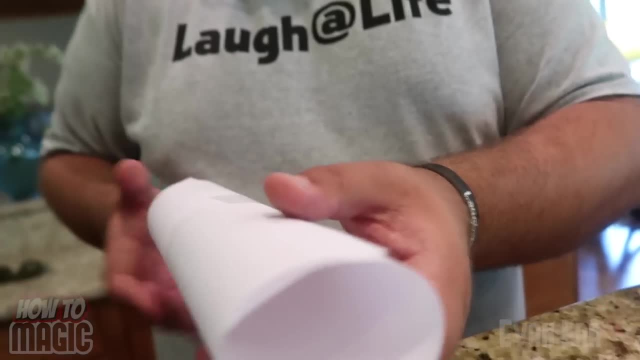 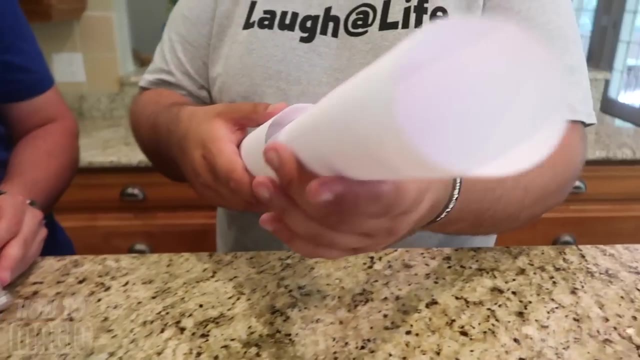 You can see this is a little smaller than the opening on this end. Hard to tell on camera, but I'll show you in just a second Tape there and another piece right there. Now that you have this taped up, this paper roll will fit inside the other one, just like this. 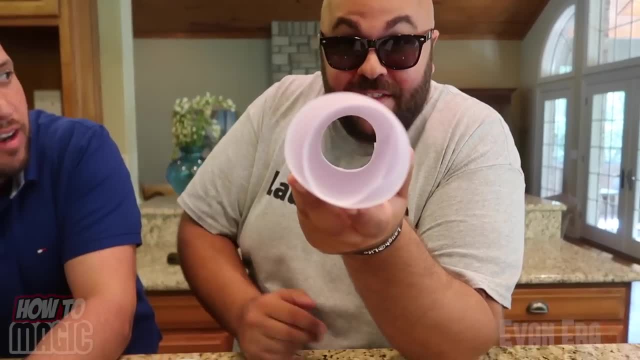 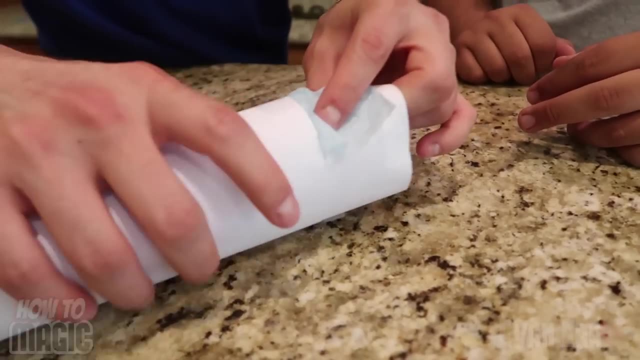 So now that they're lined up on the back end you have a secret compartment that's been formed inside the paper tunnel. So now you can take the tissue paper, wrap it around the smaller one. You're stuffing the tissue paper in bingo, bango, bungo. 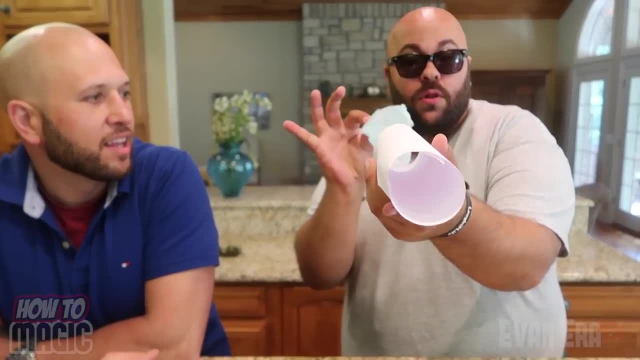 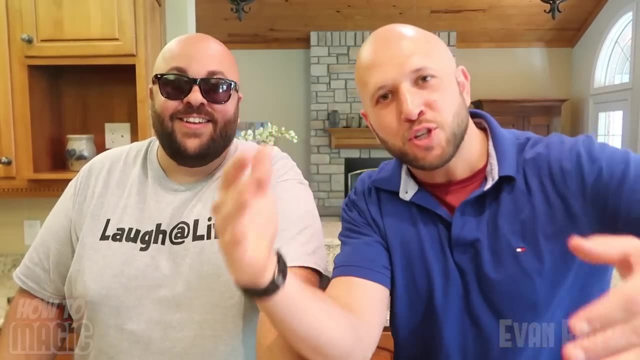 Now you can show an empty paper tube and magically pull a piece of tissue out of it. Wow, Super easy, and you can do it at home right now. That's a good one, And that's how you do the magic paper tube trick. 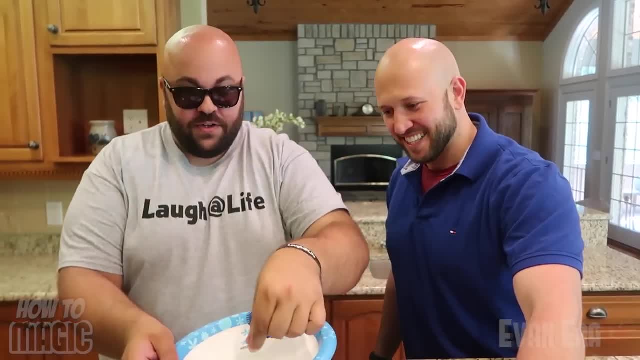 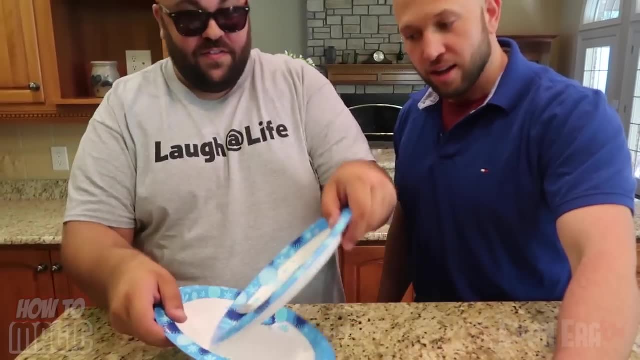 This is the magic multiplying money trick. Okay, so you're going to take a quarter. sit it right down here on a paper plate. I'm going to take another paper plate like this. You see, the quarter multiplies again. just like that. 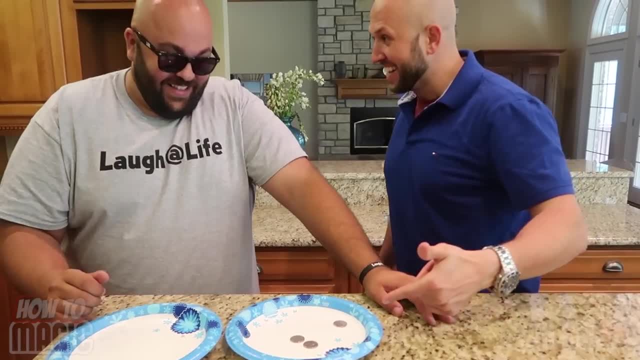 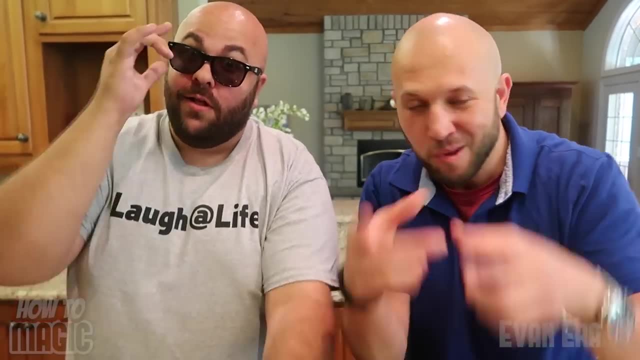 Dude, let's get more plates. I think we can make a whole dollar out of that. How did you do it? I'll show you how it's done right now. All right, here's how it's done. I'm about to reveal the secret. 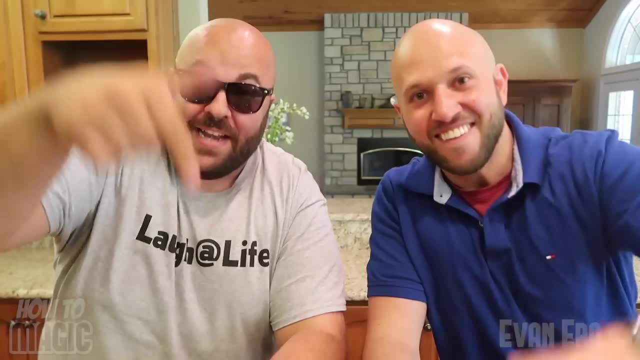 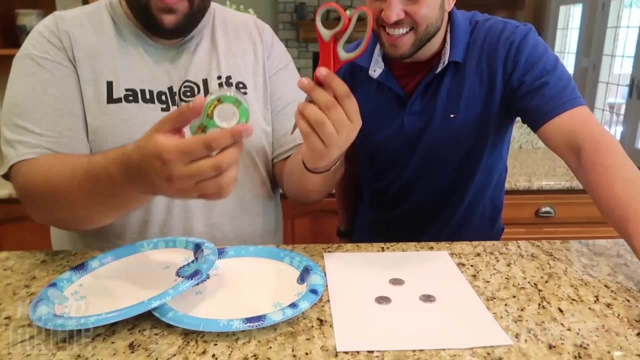 The secret to this trick is extremely simple, and I'll teach you how it's done right now. Okay, here's the explanation to the magic multiplying money trick. I love multiplying money. Here's what you need: You need some tape, You need some scissors. 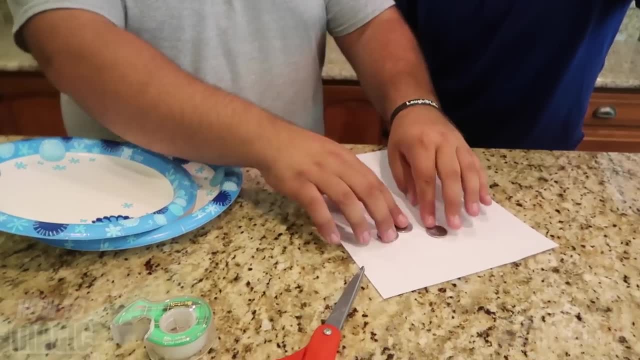 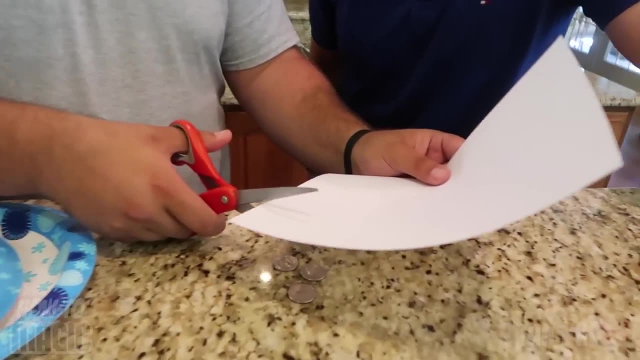 You need a couple paper plates. You need three quarters or three coins, They don't have to be quarters. You live in a different country, different currency, You can use different currency And you need a piece of paper. So, first step, you're going to cut out a little square of paper like this: 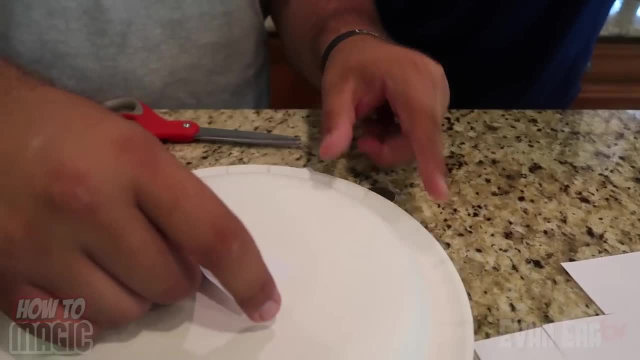 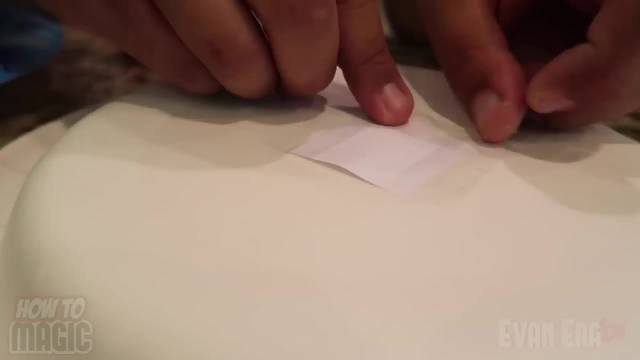 and another one the same size. All right, so your first step is to take a little square of paper. You're going to tape it onto the bottom of the plate. It's like a little pocket. Yep, exactly, And one across the bottom, just like that. 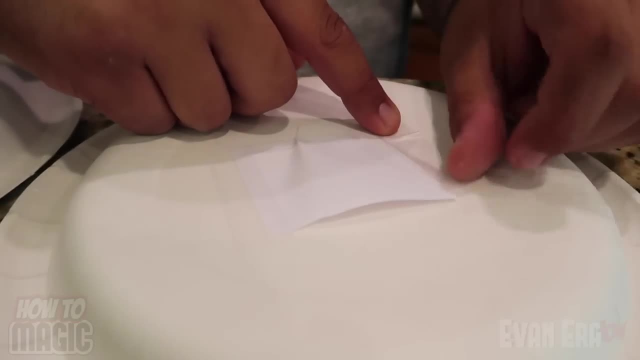 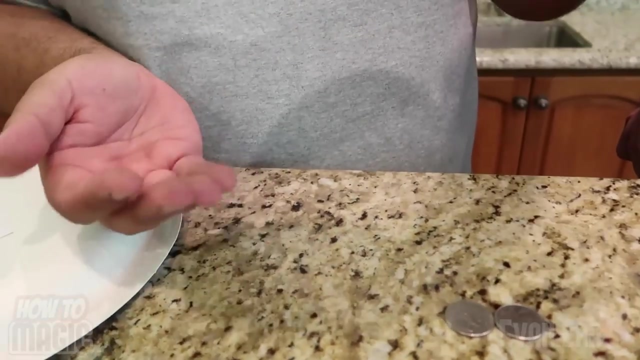 And we want to leave this side open so that the coin can fall out of it. We've got to tape down like that And now our quarter can go right inside. It can seal underneath the plate, But when we kick it sideways, 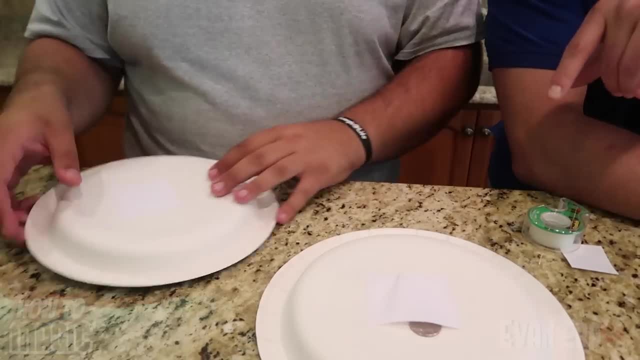 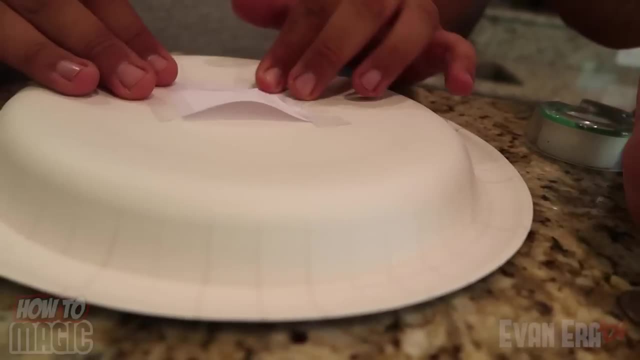 the coin will fly out onto the other plate. That's key. Now, where do you buy these magic money plates? You can buy paper plates at any grocery store. Tape that in place, and now your coin should comfortably slide in. 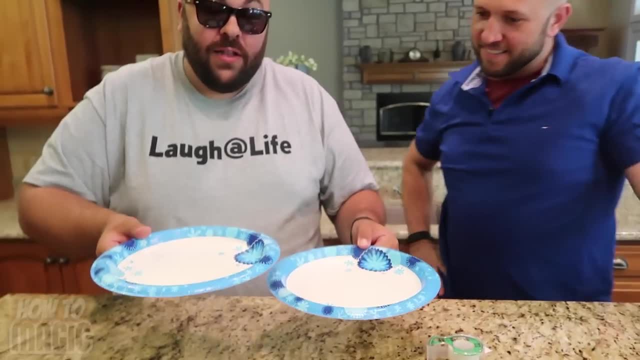 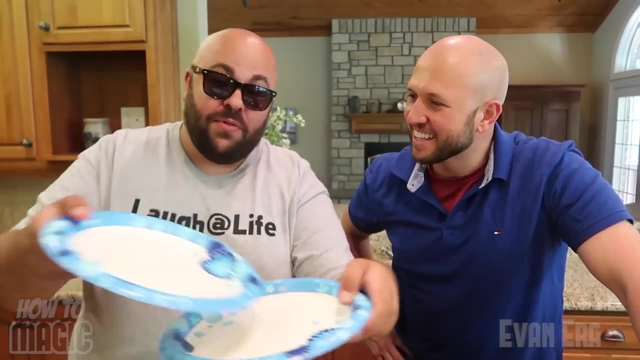 And slide out. Once you have the coins loaded in, you can then hold them horizontally and the coins won't fall out. Don't let them see the bottom of the plate. Precisely, You want to make sure the opening is lined up over top of the other plate. 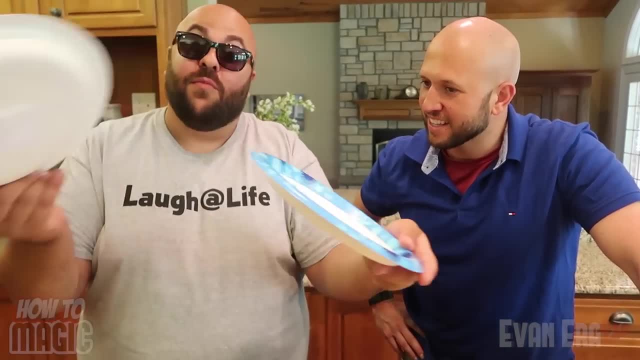 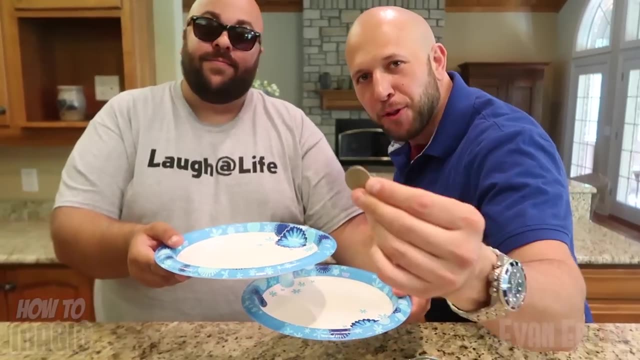 so that when you kick it sideways, the quarter falls out on top of the other plate. Looks like it's multiplying the money. So you've got it set up: One quarter here, the other quarter on the other plate And then the magic quarter that's going to multiply all the money right on top. 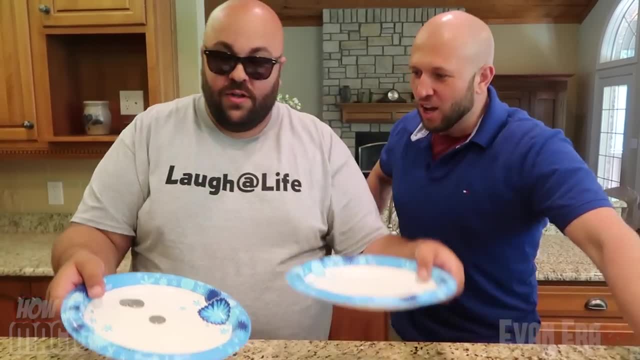 Boom. So as you kick it over, Woo, 50 cents. We need more plates. Into three: We need more plates. Let's get more plates. We're making money over here, boys and girls, We're making money. 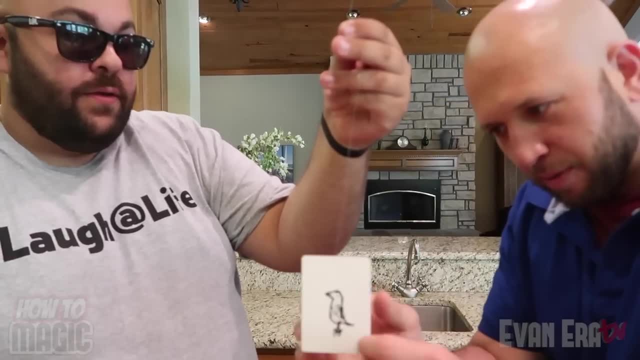 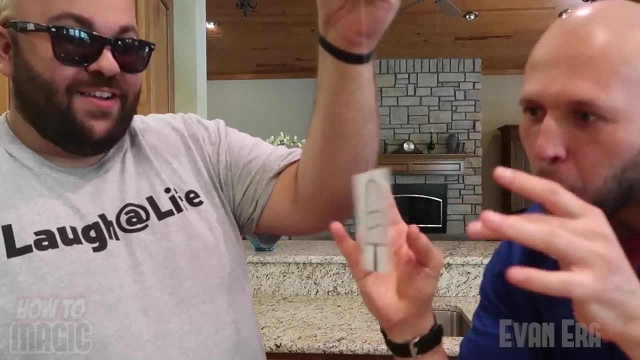 This is an easy optical illusion you can do at home. Check it out. For this magic prank. I'm going to make the bird in the cage by just rubbing my hands. Isn't that cool, Okay? so here is what you need for this amazing magic trick. 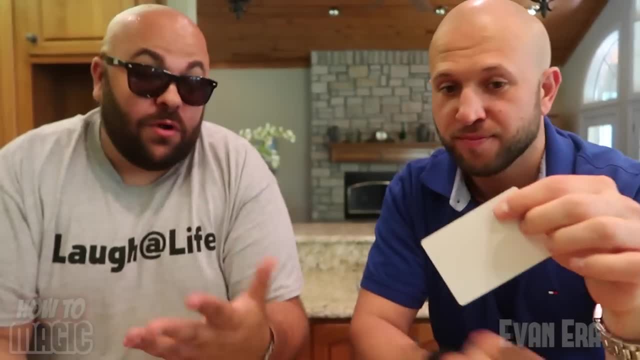 You take a blank card, Blank on both sides, Just like a normal bicycle card, but it's blank. The reason we need it blank is because we're actually going to take a marker and we're going to draw on either side of it. 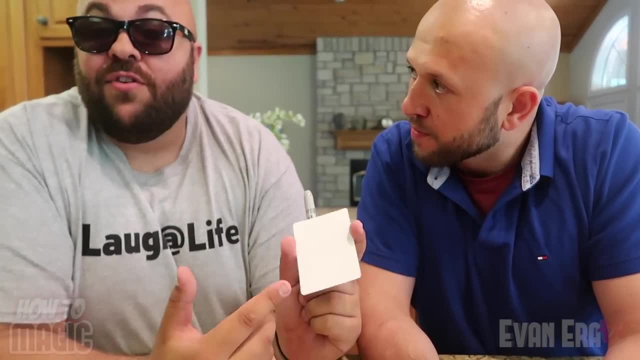 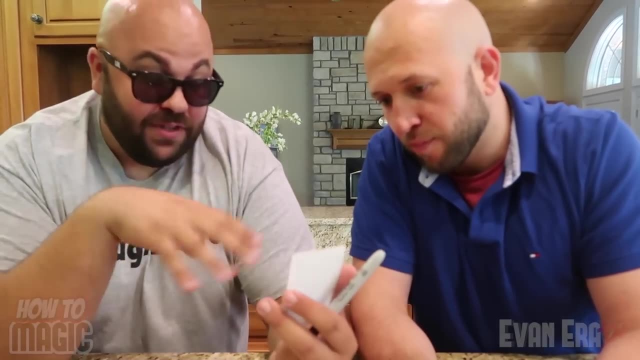 The cool thing about this is it's like an optical illusion. The bird is actually never in the cage at all. It never really happens. It's just because the image is spinning. It looks like they join together and the bird becomes like inside the cage. 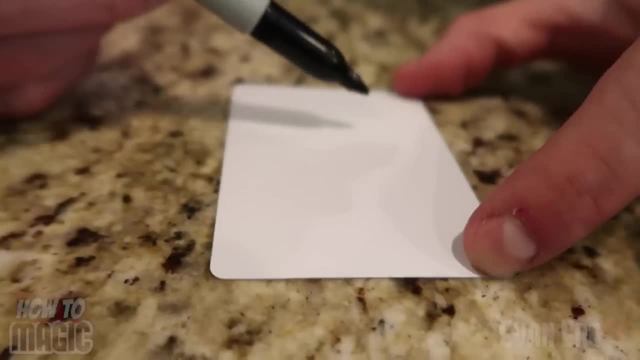 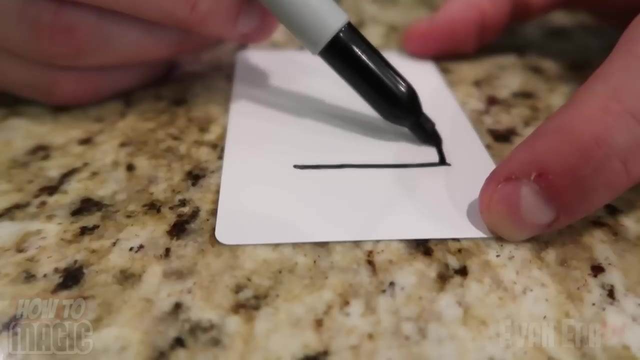 It's really cool. Let me show you how to draw it. Dennis is going to draw our bird cage for us. If you guys ever watched Looney Tunes or anything, this is like the bird Tweety Bird with sleep. You just put the bottom and then you come up to the top, like that. 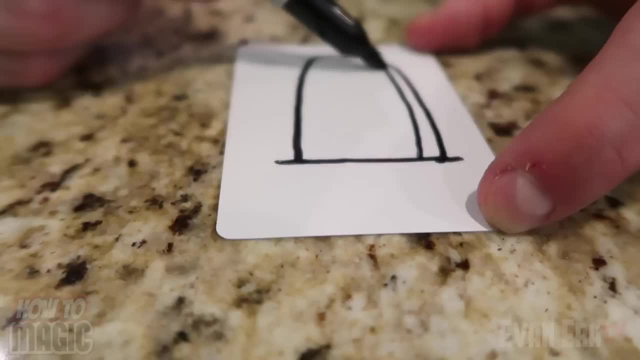 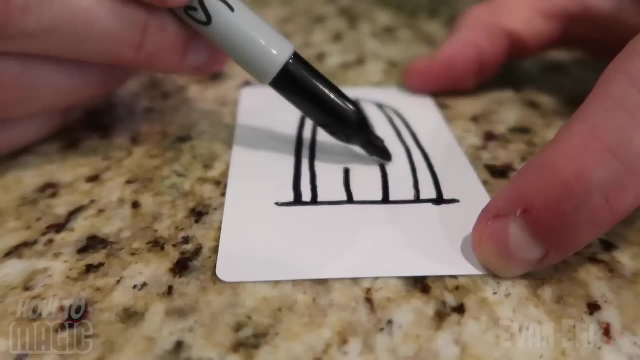 Uh-huh, Yep, and then a little stand there like that, Yes, like a jail. Then you leave a spot for the door. Oh, look at this folks, Look at this How to draw, How to magic. okay. 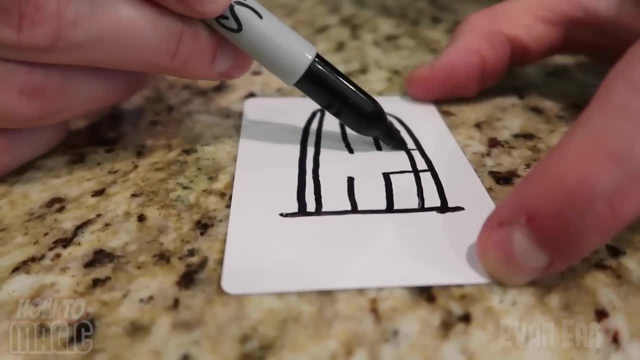 And then we'll just do the door like this: Happy little door, Happy little door, This is a happy door. You go in and out of this door, You draw a little stand at the bottom. Oh yeah, of course, of course. 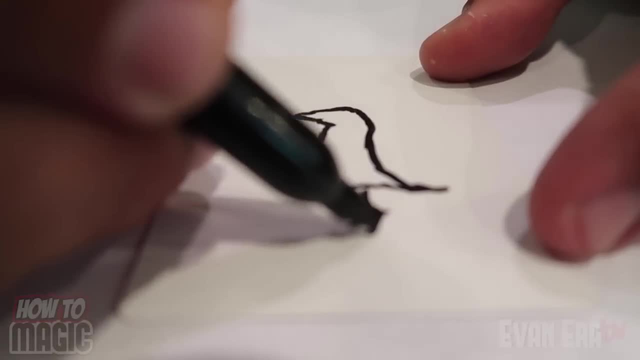 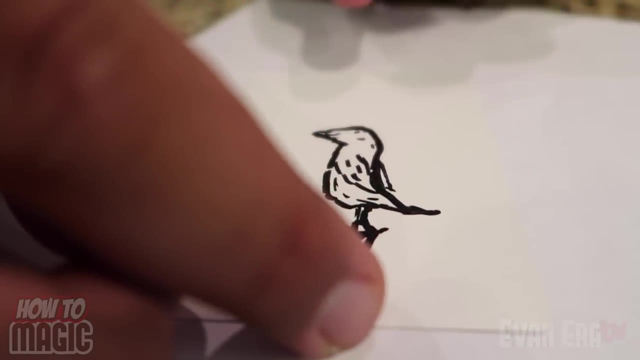 Okay, and I'm going to draw our bird on the other side. Aw, You made a great little happy bird. What was that? That's great. And your next step is to punch a little hole in this side of the card and this side of the card. 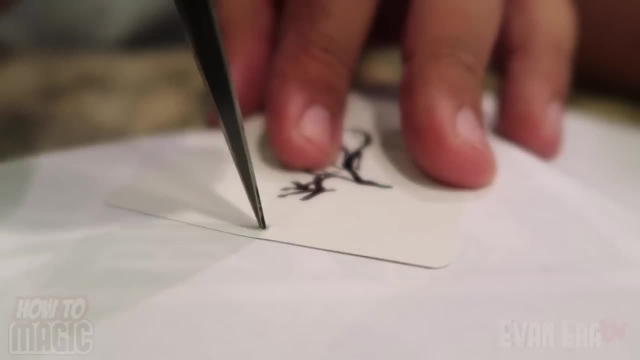 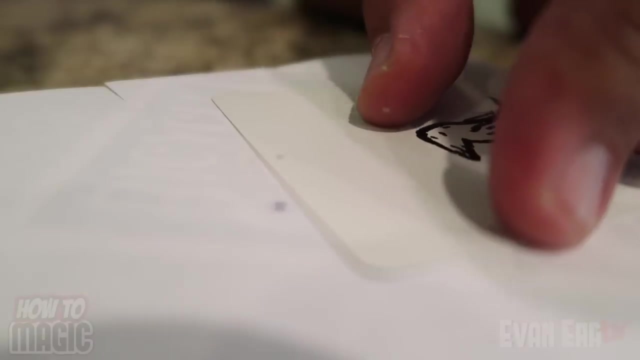 so that you can string it up on some fishing line. You got it, boy. Now do the same thing on the other side. Now do they have to be exactly lined up. You want it to be pretty close to lined up, All right. so now that you have the little hole punched in the card, 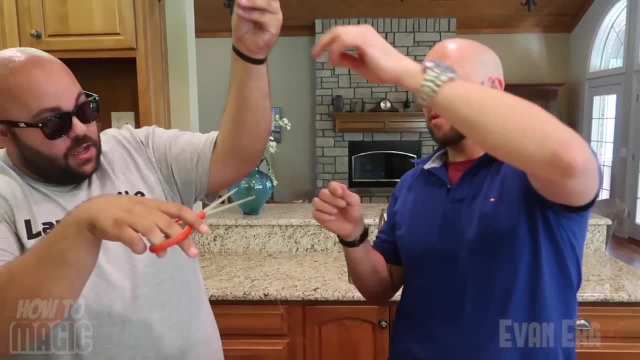 we're going to string it with our fishing line. Take about a foot of fishing line on each side. Take this and tie it on. It reminds me of sewing class when I was in like elementary school. All right, so now how's this work? 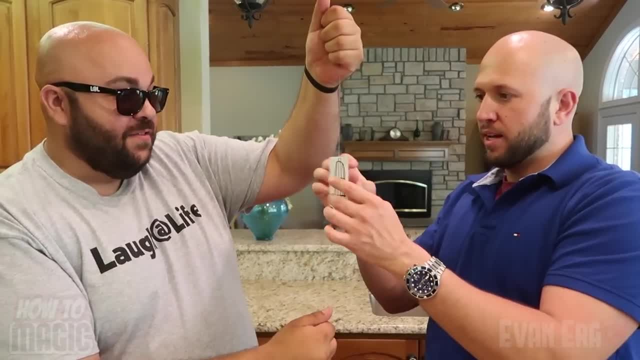 We just twist it up. So we're just going to hold it by either end and we're just going to twist it up. that's right. I like the idea of this. It's actually called a thaumatrope. This is a classic magic trick. 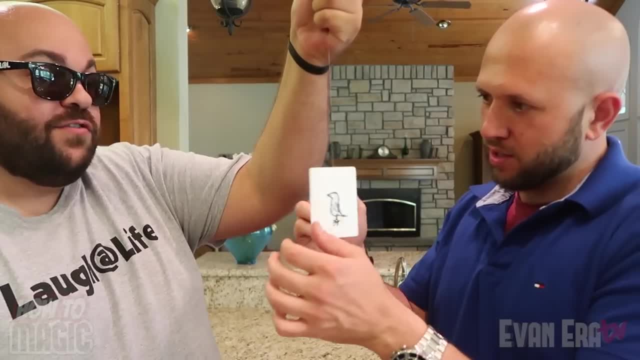 I mean, I'm no magician or anything, but you don't have to use fishing line, right? No, you can use string String. actually would probably work better than fishing line, but all we had was fishing line. Let's see if this works. 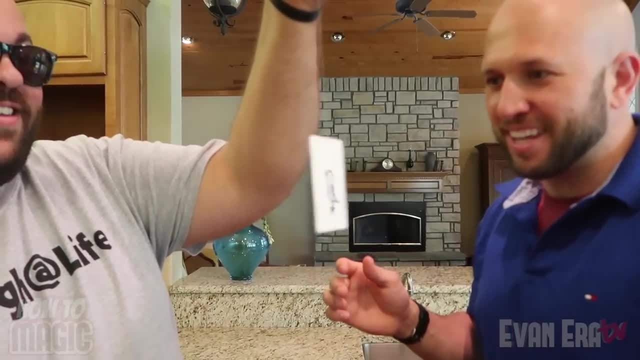 Ready to let it go? Uh-huh Whoa. looks like it's in the bird cage, but it's not. So this isn't limited to just a bird in a bird cage. You can do a dog in a dog house. 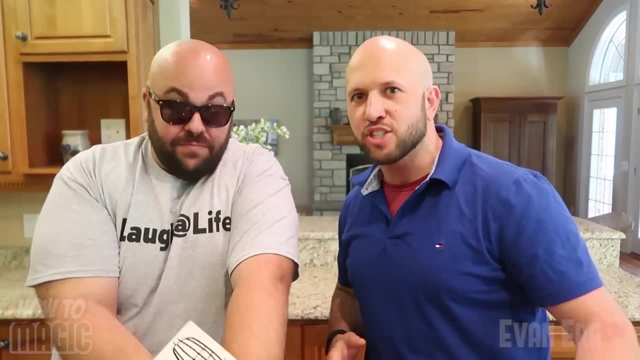 You can do a prisoner in a jail cell. You can do all kinds of things. Just use your imaginations and apply a little magic and you'll wow your friends and family. Super easy magic trick that you can do at home with no practice at all. 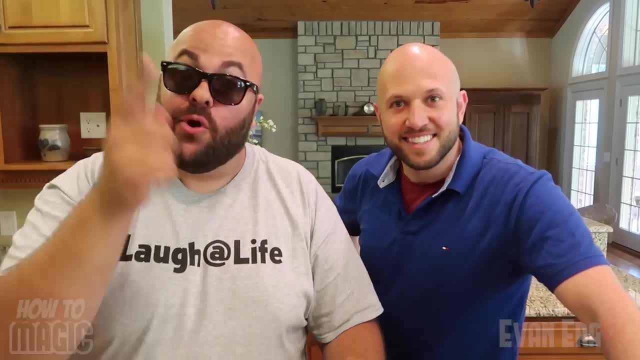 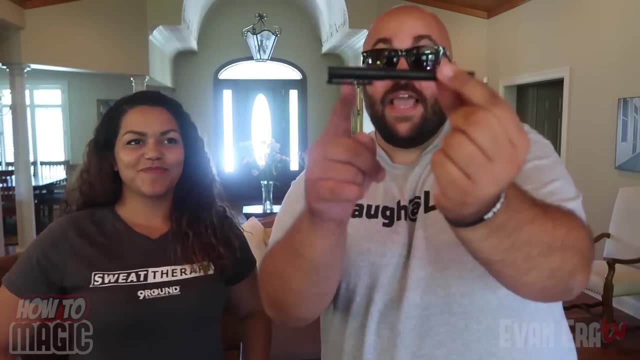 I had this the first time I ever did it in school, And that is how you do the magic bird in the cage trick. This is a great school magic trick you can do. All you need is a pen. Check it out. OK, so you're going to take a pen. 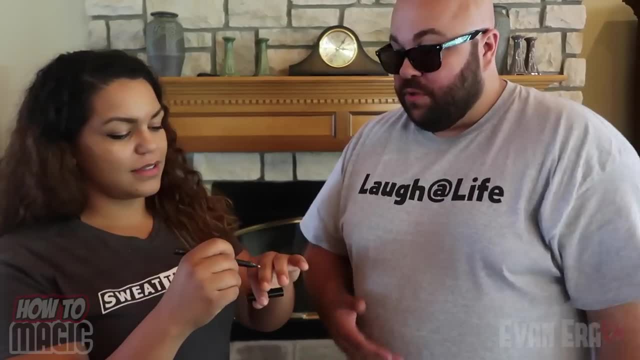 As you can see, it's a normal pen. Nothing tricky about it, Normal enough. put the cap on: Oh, just wrote it myself. Yeah, it's normal. It's normal. All right, watch, I'm going to take the pen like this. 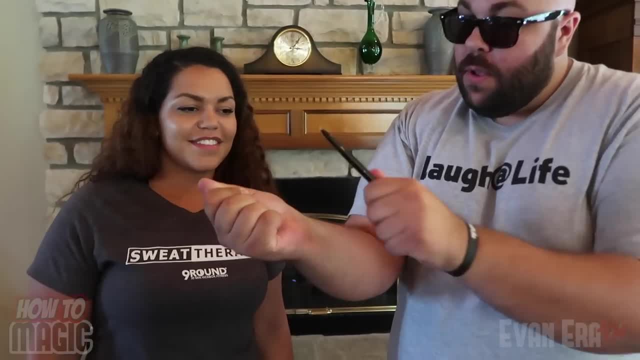 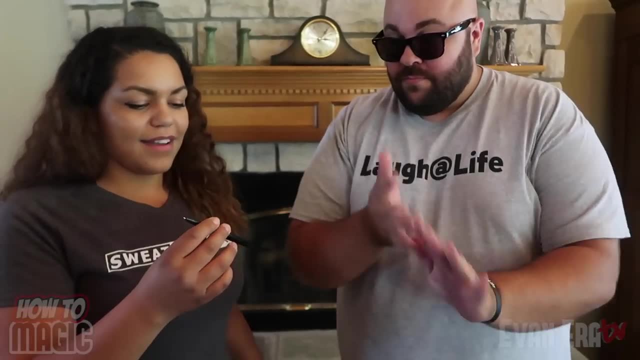 remove the cap in my hand and look OK, And just rub: Yo wait, how did you do that? That's cool, That's magical. You want to check it out. You want me to check out the feet and the nose, don't I? 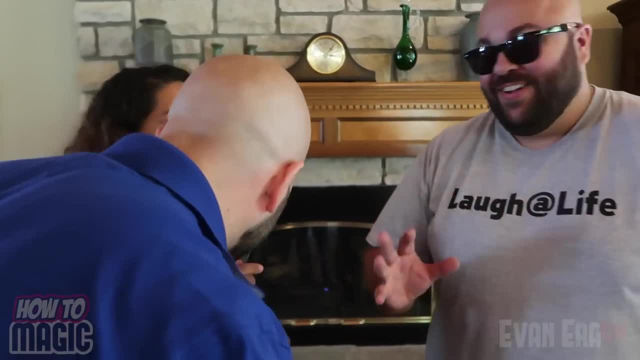 Reveal it, Reveal the secret, And you have no sleeves. That's really cool. Here's the secret. OK, here's the explanation to the magic pen trick. So the secret to this: this is actually our magic pen, available at howtomagicshopcom. 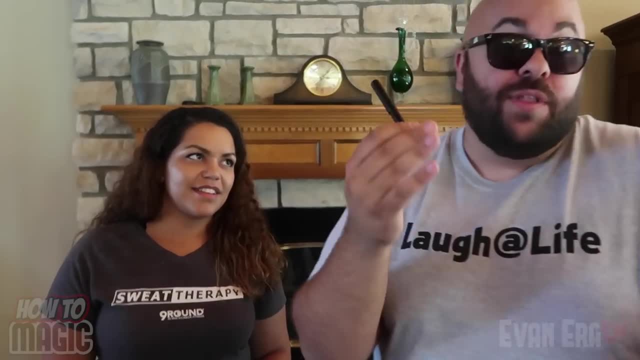 So the cap goes on the pen like this. This is all sleight of hand. This has nothing to do with the pen. You can do this with a pen at home too. So the cap's on the pen, You're holding it like this. 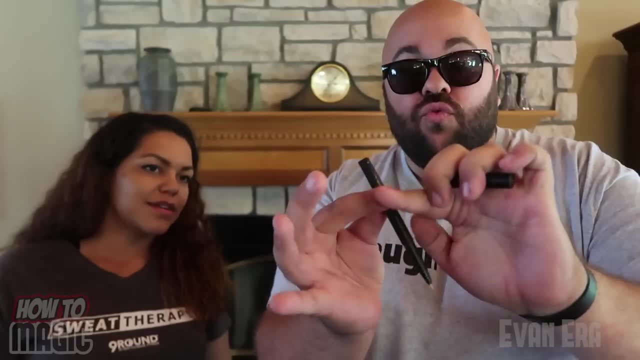 And all you're going to do is slip the pen top into your hand as you rotate the pen like this and grab it to make it look like you're pulling the cap off. Do the slow-mo. You're actually retaining it right here. 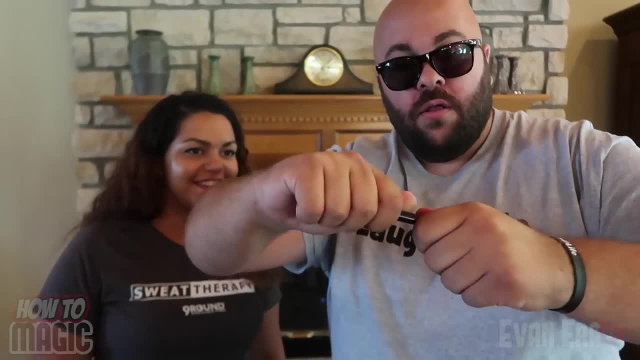 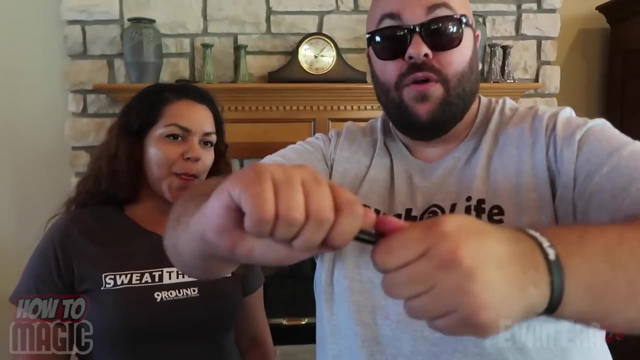 It's here and like that. So it's boom, concealed in your hand. You're sliding that out as you rotate it around, And now you're grabbing and making it look like you're pulling the pen top off. This is all acting. 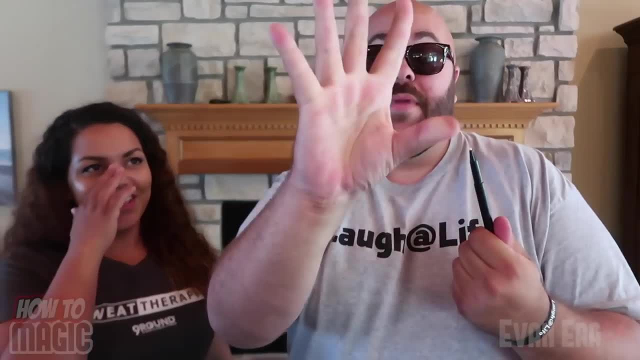 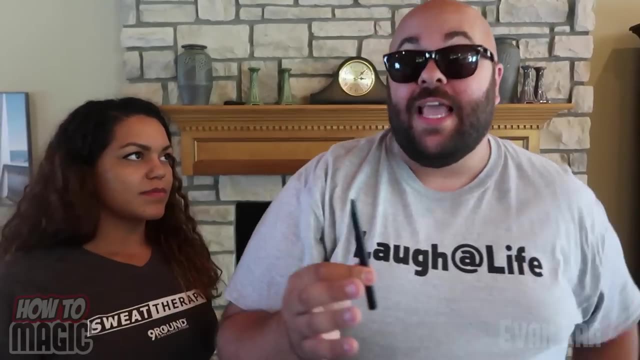 Make sure you sell this, that the pen top is actually in your hand, Make it disappear. You're looking for the cap And then, when they are looking at this pen and you hand it to them, you're going to drop this hand to your side and dish the. 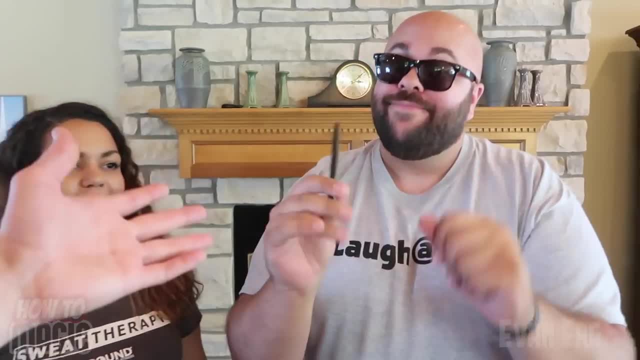 cap into your pocket and just hand right back up into their field of view. Oh, oh. and then that's when you can say: now, the magic pen is behind your ear, Okay, so you're going to take a pen like this and you're. 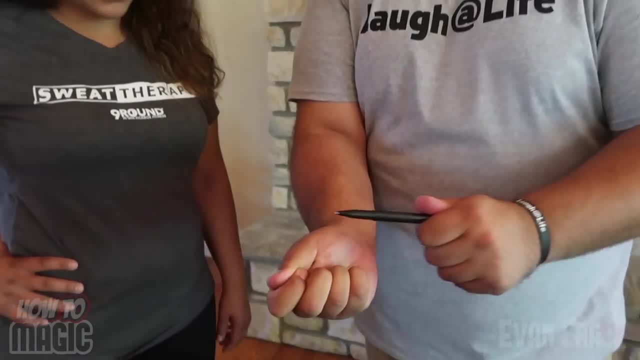 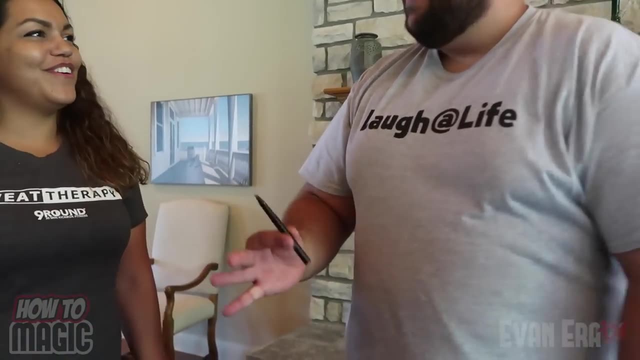 actually going to remove the cap in your hand. give it a rub and it'll disappear, just like that. You know where it went. It's actually behind your ear And that is how you do the magic pen. It's called the magic disappearing pen cap. 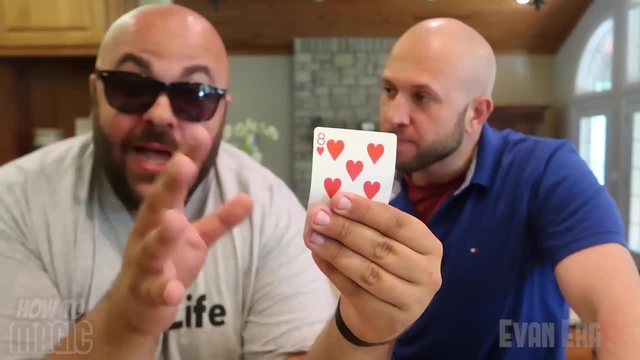 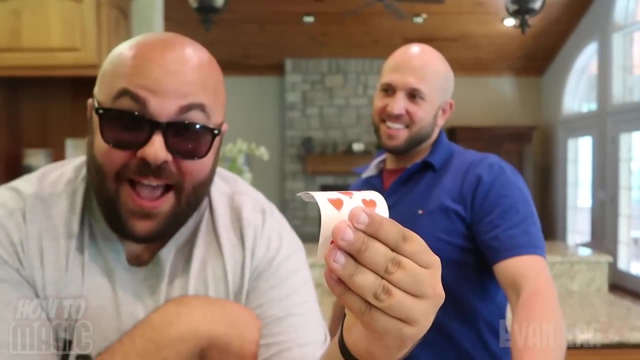 For this one. you're going to do something impossible with the playing card. Okay, so you're going to take a card from the deck and watch. Oh yo, that's awesome. You can magically bend and hack. Here's the secret behind this amazing card trick. 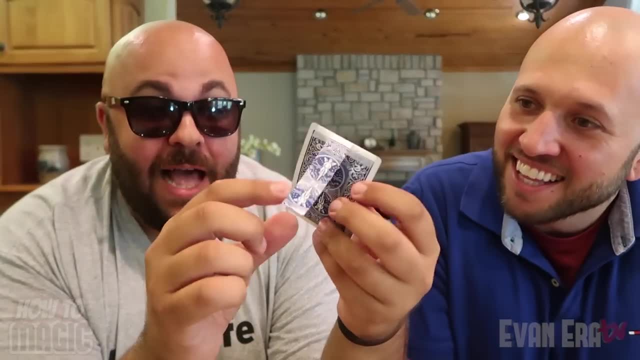 Check it out. Okay, here's how it's done. It's super easy. You just take a little flap from an extra card. That's good. All you need is a deck of cards, pair of scissors and some tape. Here's how you set it up. 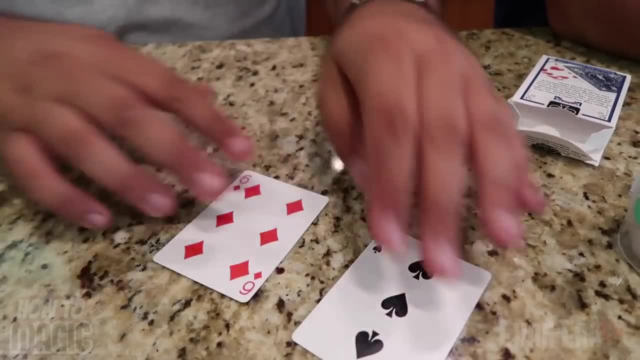 So you're going to remove a card from the deck- any card you want- And then you're going to remove an additional card, It doesn't matter which one, Start out cutting a piece of card just like this. So three cuts like that. 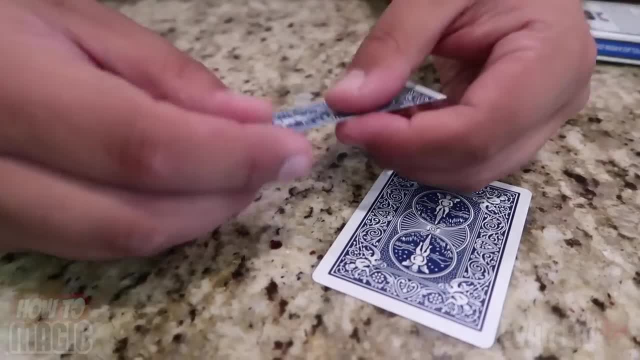 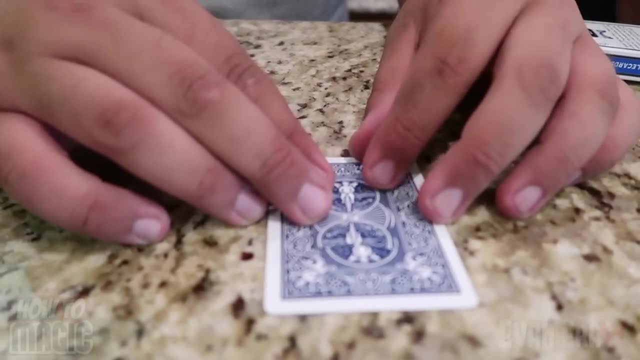 Yep, and you just want this middle piece. You can get rid of these other two pieces And now you're going to tear this across the top about three quarters of the way up. Discard this, You don't need that. All you need is this piece, right here. 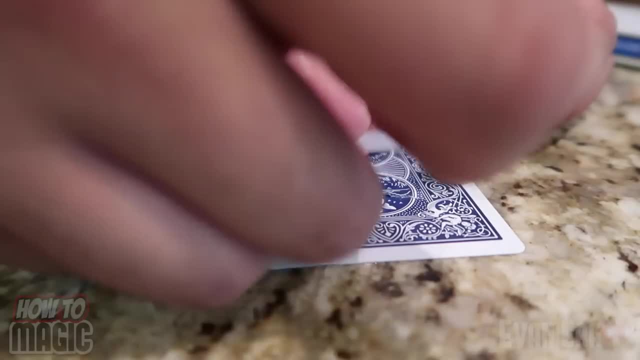 You're going to line that up on the back of this card so that it looks seamless. Now you're going to put a piece of tape right along the top. Make sure it's lined up. Now you can show this pretty openly on the back, as long as you keep it quick. 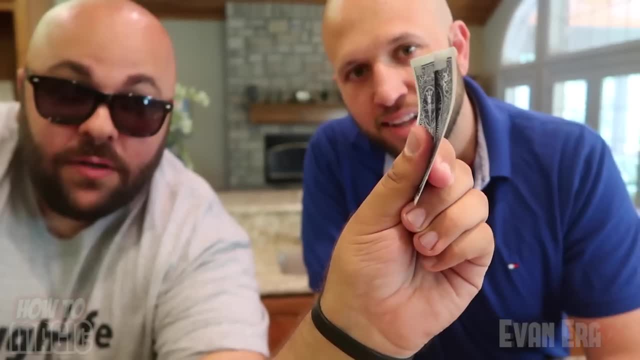 You can hold the card like this and as you pull your thumb down, it's going to bend. Do you sell magic cards on your website? I do. Oh, that's awesome, dude. You should customize them to say Evan Era. 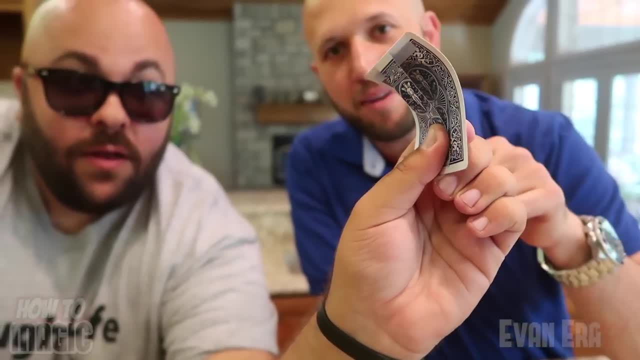 That would be cool. If you guys want to see custom decks, let me know. Let us know in the comments below. if you want to see custom Evan Era decks, You just pull your thumb down and the card will magically bend, like that. 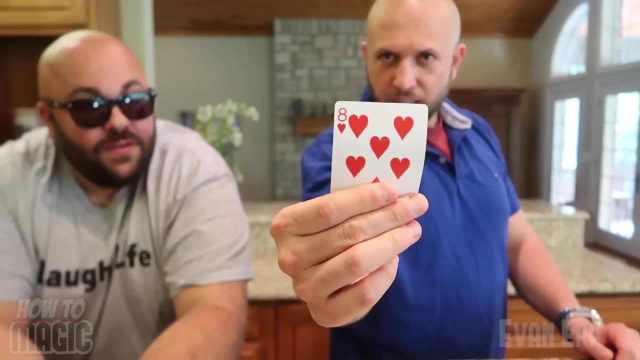 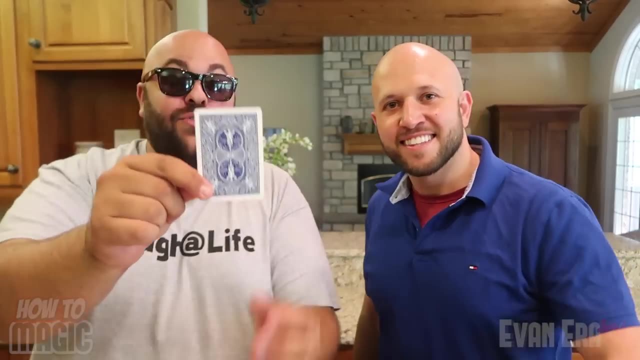 Super easy. Let me try School trick. buddy, You'll take my notes if I can make this card bend. Yes, Look at my magic face And that is how you do the magic bending card trick. Wow, Okay, This is a fun magic trick that you can do at home. 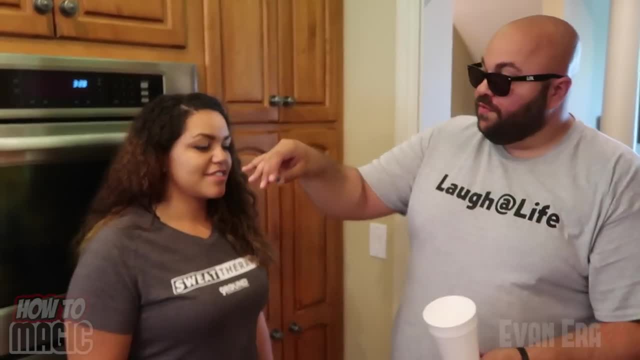 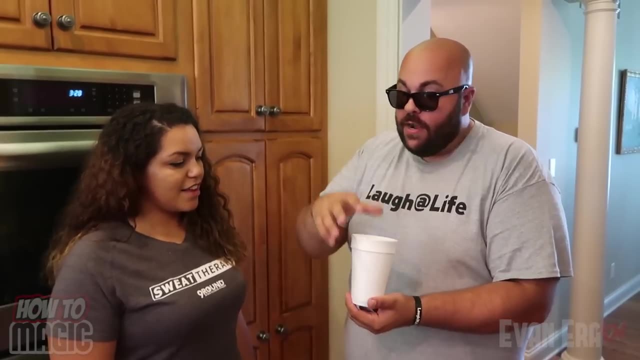 With a cup. Okay, Veronica, I have a cup here and I have a couple of marbles. If you would check those out for me, Real marbles, right? All right. So I'm going to set them inside the cup, just like this, and go right inside. 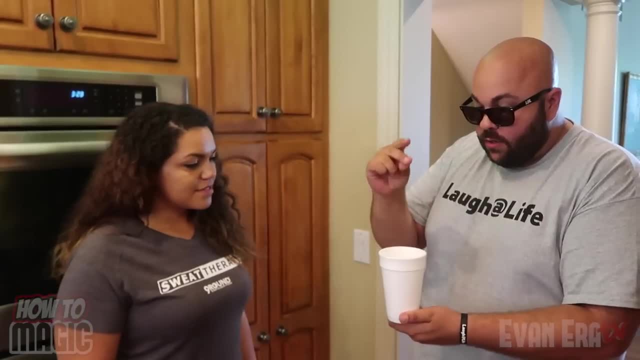 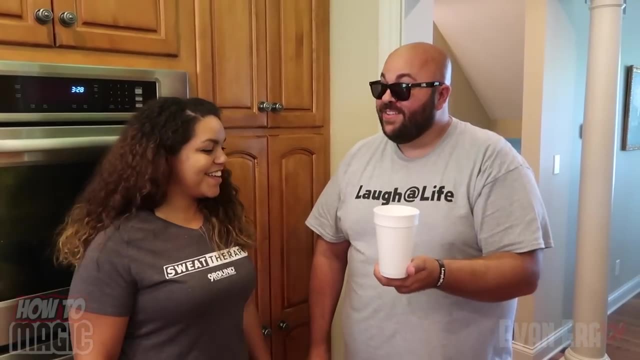 And now watch. If I just give the cup a magic wave, look Yo, I love that trick. Do it again. The marbles magically disappear. I want more. Do it again. That was awesome. Okay, Here's the secret behind this crazy magic trick. 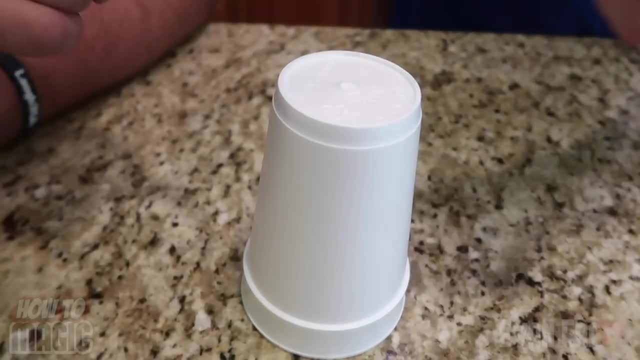 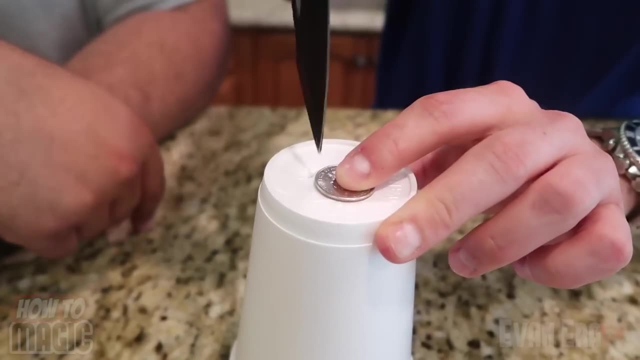 So the first thing you need is a cup. Your first thing you need is a cup. Your first step is to cut a hole about the size of a quarter in the bottom of the cup. So maybe get a parent's help and cut a hole right in the bottom of your cup. 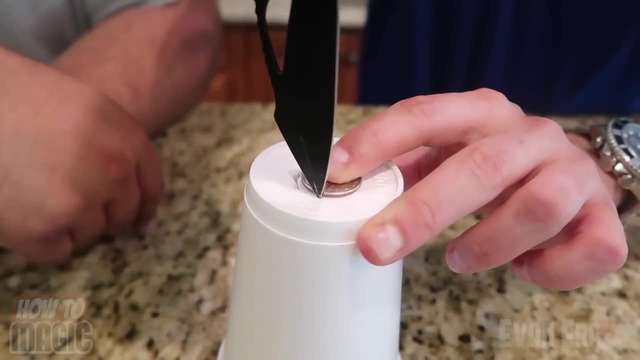 Paper cup would probably work better, right? Yeah, You probably want to use a paper cup, but we're going to use styrofoam because that's all we've got. So once you've got your hole cut in the cup, your next step is to take a piece of white paper. 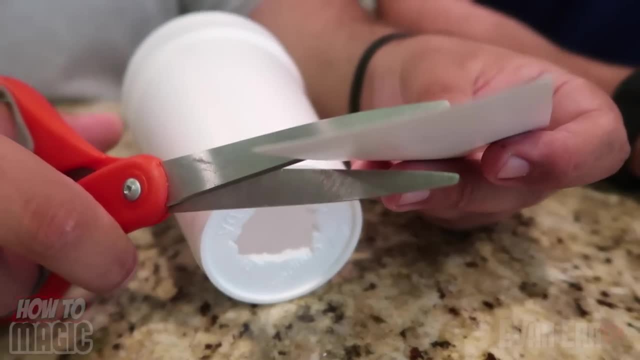 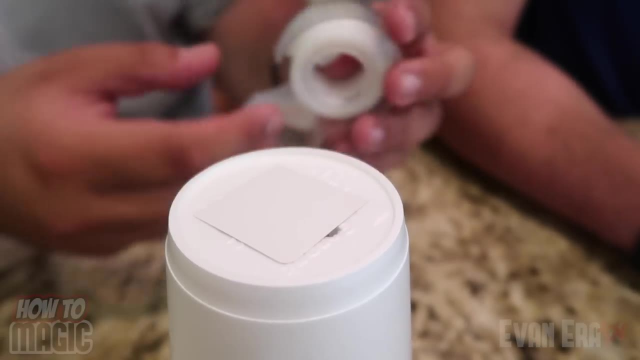 In this case, we're going to use a white card And we're just going to cut a little square of it off And you're just going to put that little flap right over the hole, like that, And you're going to put a piece of tape on one side to kind of create a little hinge for it. 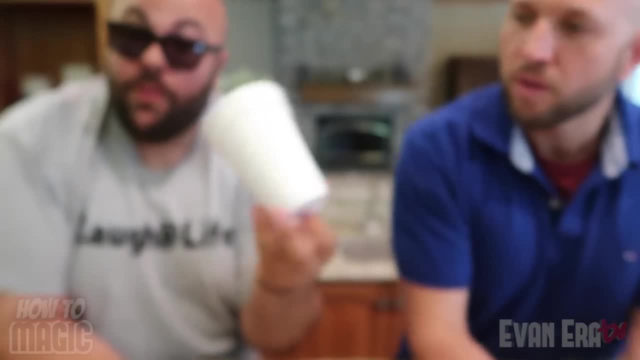 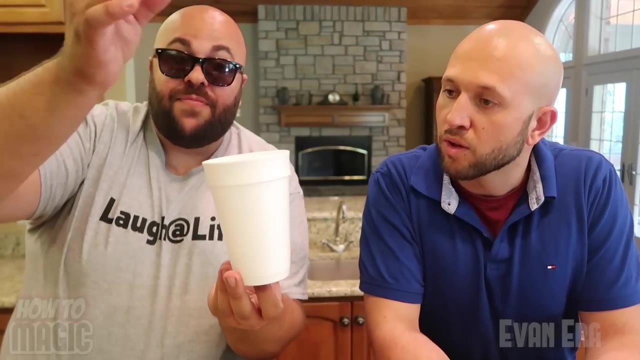 Put our tape on and create our hinge. Now, when we hold our finger over it, we can briefly show the inside of the cup is empty. So now the flap creates a closed bottom on the cup when you hold your finger over it, so that you can drop things inside. 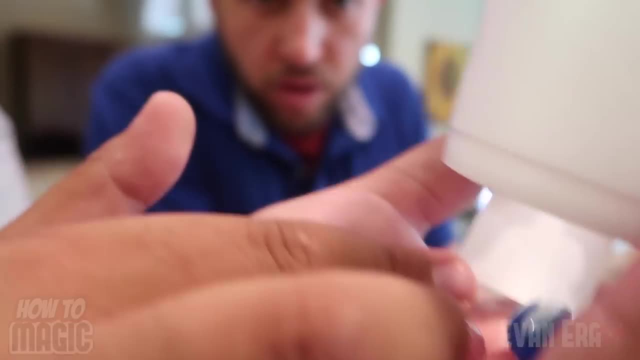 And then, when you let your finger off the flap, the marbles will roll out into your hand. You can palm them. And then, when you turn the cup upside down, nothing comes out. Oh, that would be cool. Looks like it totally disappears. 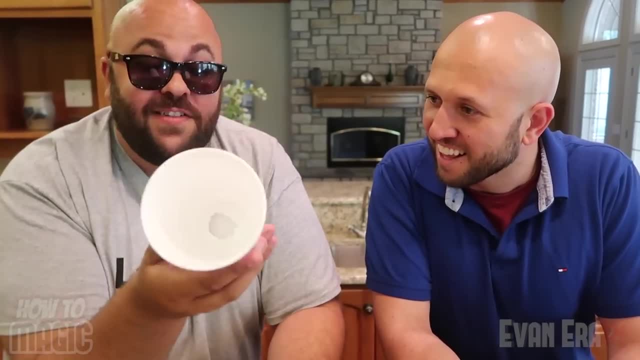 Really easy. So practice this at home. Make yourself a disappearing cup. That's a great magic trick to pull off at lunch For sure. So as far as stuff that you drop in the cup, it doesn't really matter as much, Yeah. 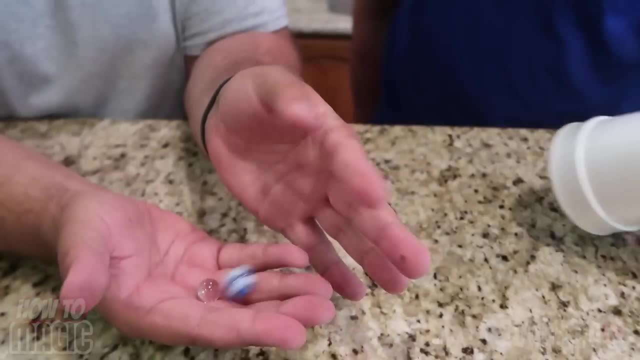 As long as it will fit out of the hole in the bottom of the cup. We have marbles because we like marbles, So you can use marbles. You could use pencil erasers, You could use coins. You could use rolled up balls of aluminum foil.